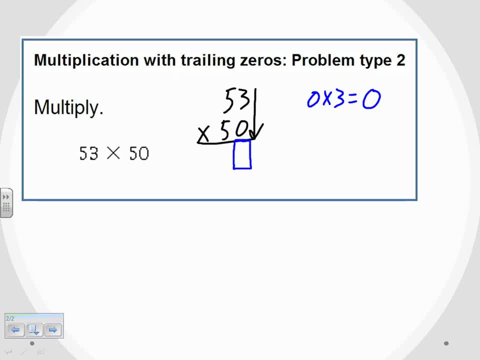 space here which is right below the zero that I'm multiplying from. is that first zero, And then I keep working to the left. That was zero times the three in 53.. I have to do the next digit, which is the five. Zero times the five. 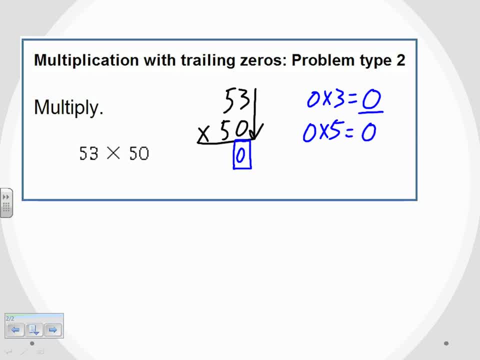 gives me the first digit. So I'm going to do that. And then I keep working to the left And it gives us again zero. So my second digit here is zero. That goes in the next space to the left. That's another zero. So I've multiplied everything in the top by that first zero. 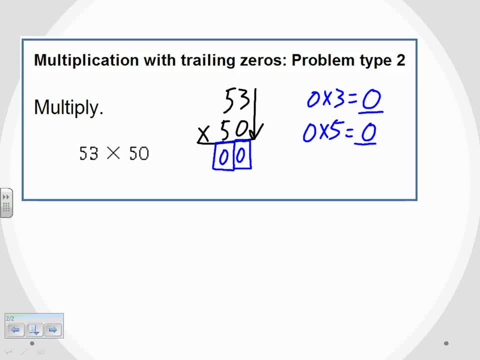 And now I need to move over to the next digit to the left, which is the five. So I need to multiply everything in the top By the five, So five. I want to start with the digit furthest on the right-hand side. 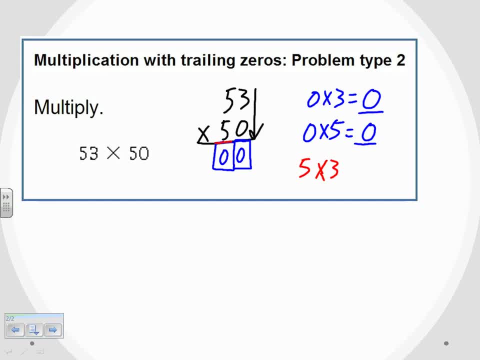 which is the three. Five times the three gives me 15.. Now, that's a two-digit number, so I'm going to have to do some carrying. But the first decision I have to make is where to put those digits. And since I'm multiplying by the five, 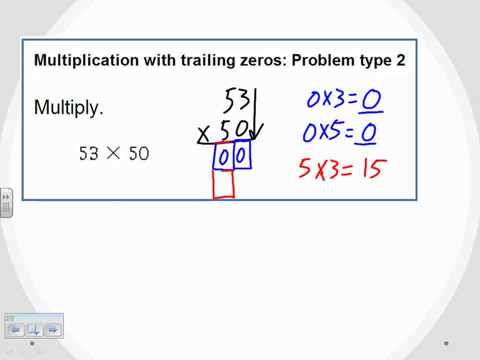 I want to start off immediately below That five. So it's kind of staggered over. I'm putting it directly below the five and I can only put the digit on the right, which in this case is also a five, That one, this one right here from the 15,. 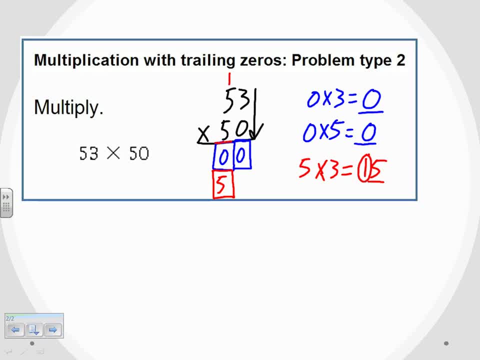 is going to have to get carried over to that next digit to the left. So we've multiplied the five times the three. We keep moving to the left. The next digit in the top is the other five. So I've got the five in the bottom times the five in the top. 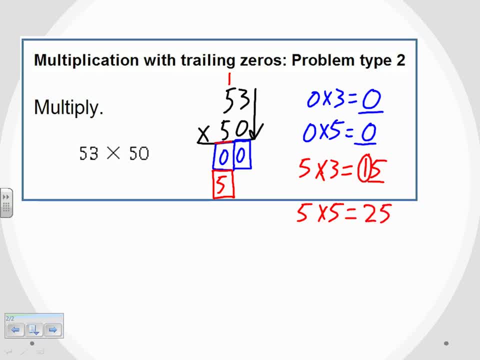 I multiply those as is and I get 25.. But I have to make sure I remember that one that I carried over and I have to add that to my 25.. So whatever gets carried is added after we multiply and that gives me a 26..